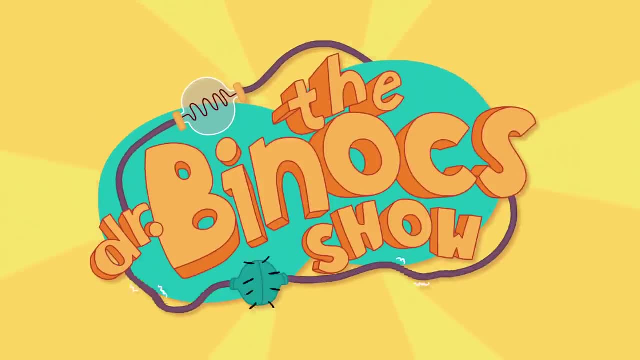 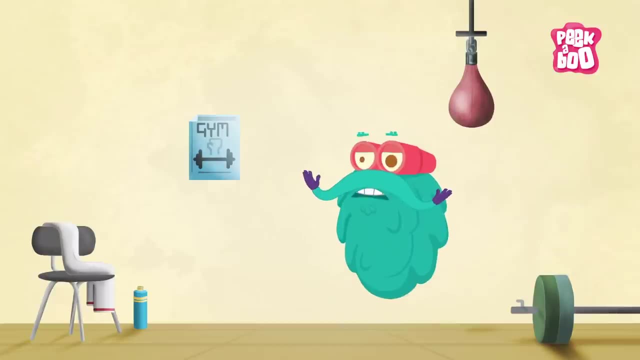 You Breathe in, breathe in out. That's what I say throughout. Breathe in, breathe in out. That's what I say throughout, whew, Hmm, Oh, so you've been watching me work out a Rather: breathe in and breathe out. whoo, this is tiring. 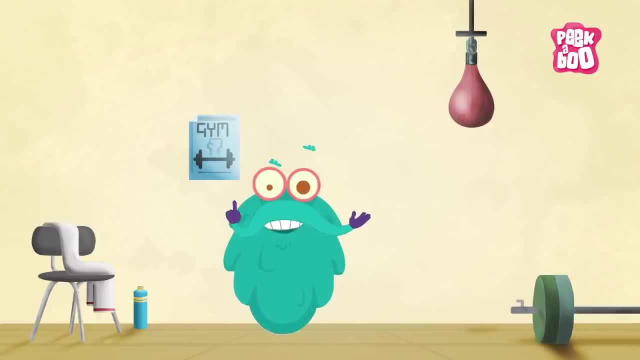 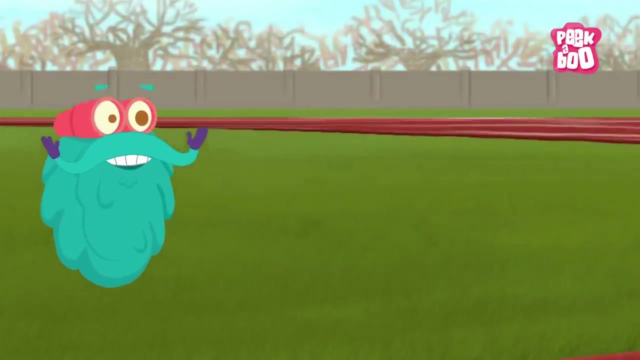 So, anyways, why don't we talk about breathing today? still can't get a hint. Still can't get a hint. Well, today we talk about the human respiratory system. Well, today we talk about the human respiratory system. Zoom in. All right, do this right now. I'm watching you. just start running wherever you are. 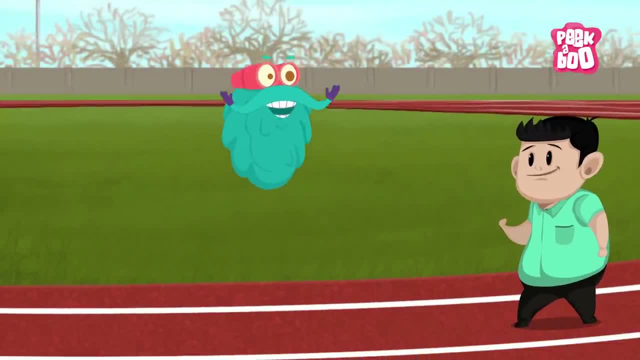 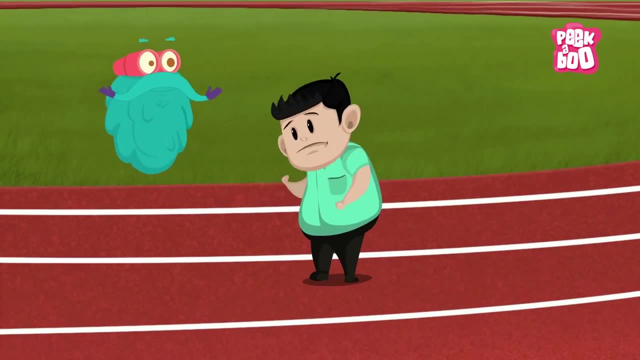 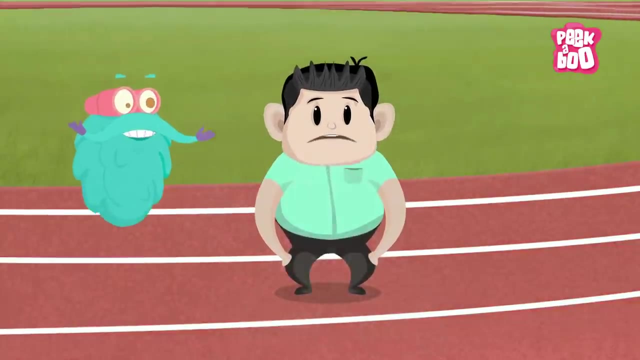 All right, do this right now. I'm watching you just start running wherever you are. Run, run, run, Run, run, run, run. Now stop. Isn't your breathing heavy? Well, that's because, right now, your body needs more oxygen to breathe, and you get oxygen from the air. 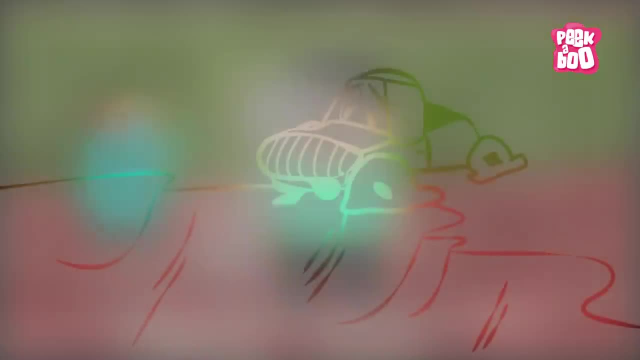 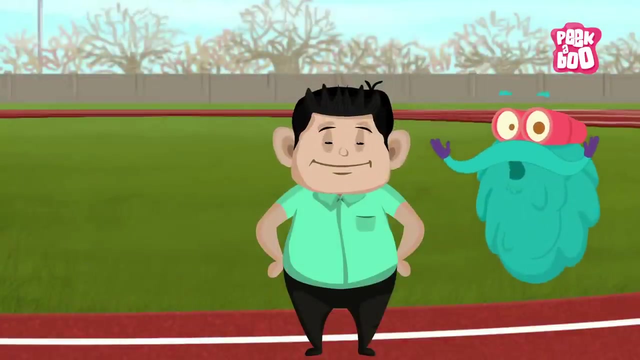 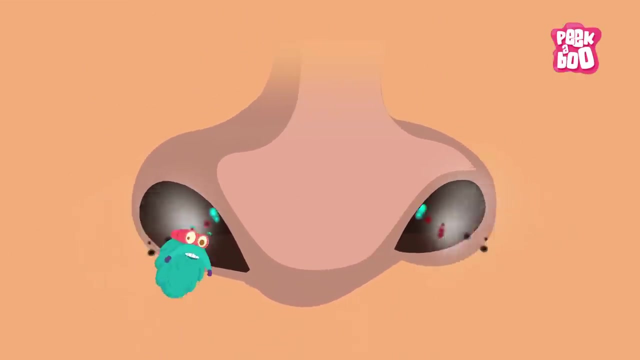 around you. without oxygen, you'd be like a car without fuel, a Waterless pool, and wouldn't that be uncool. one of the major reasons why you're alive is Oxygen, so take a deep breath in. When you breathe in, you take in oxygen present in the air. 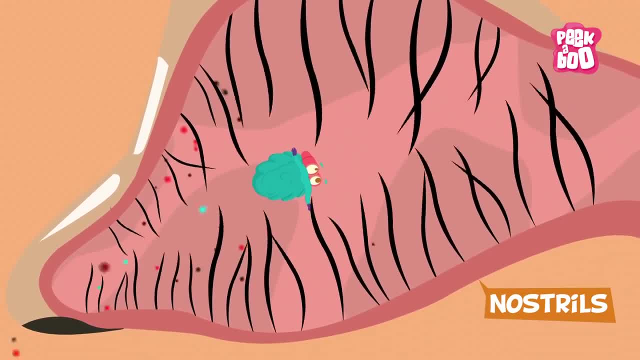 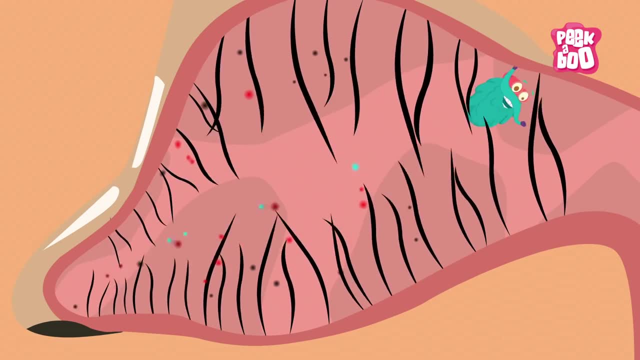 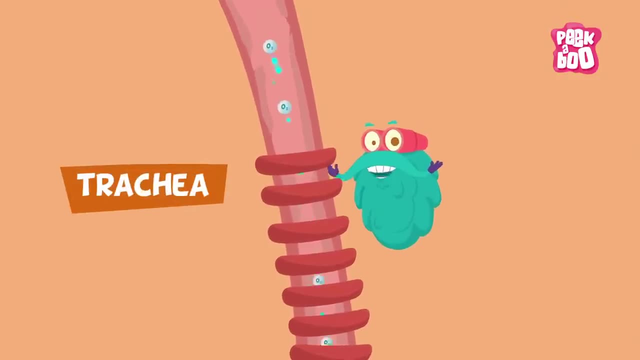 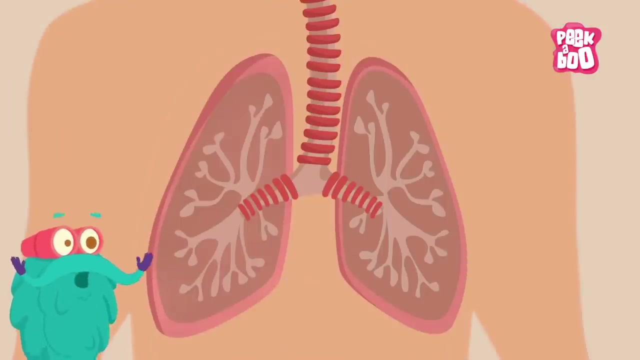 The air then passes through your nostrils. There are tiny hair present in your nostrils that obstruct All the dust particles. then the air travels to the windpipe, also called the trachea, also called the trachea, Which filters the air inhaled. The trachea branches out to two tubes called bronchi. 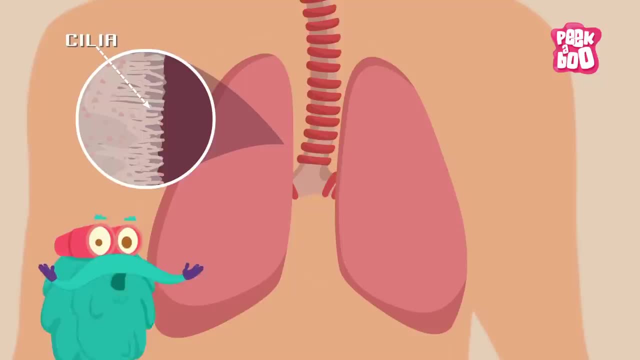 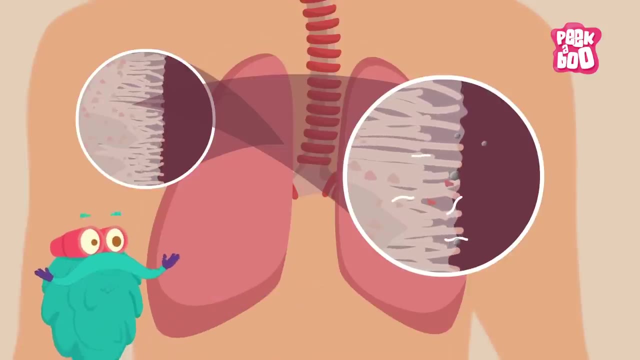 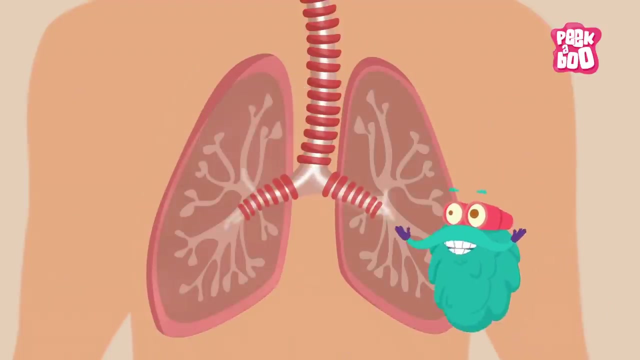 Where tiny hair called cilia move back and forth, moving the mucus. inside. The mucus is a sticky substance that collects germs and other particles that might harm the lungs. the bronchi then carry air into each lung. the right lung has three lobes, whereas